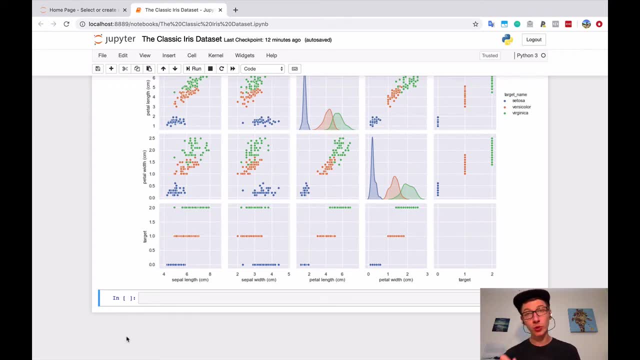 To prepare for modeling. one of the most important parts about data science and machine learning and modeling is that you always want to put aside part of your data to evaluate your model on. in the very end, You always want to- and actually even more important than that- is this concept that you always want to- evaluate your model on data that was not seen while you were training your model, while you're fitting your model. 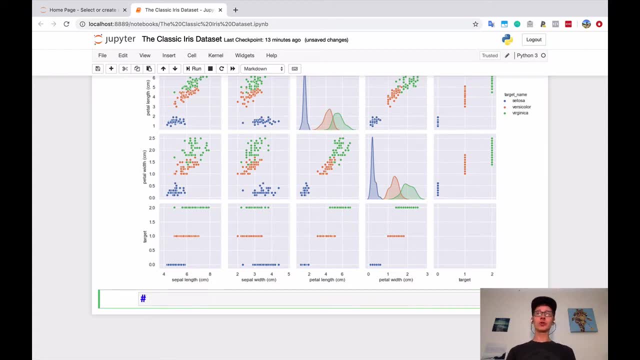 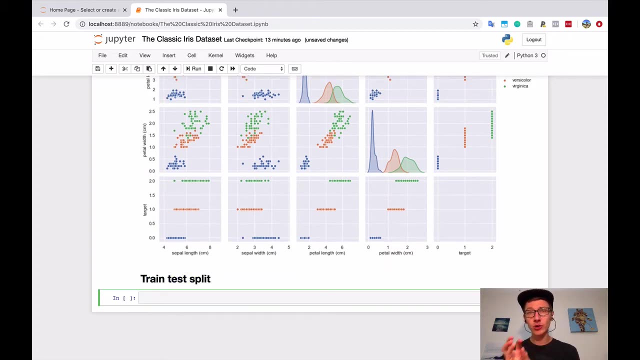 So the way that we're going to do that here, we're actually going to do it a couple different ways, but first we're going to create this thing called a train-test split, And this is setting aside a little piece of our data for the very, very end, to evaluate our final model on 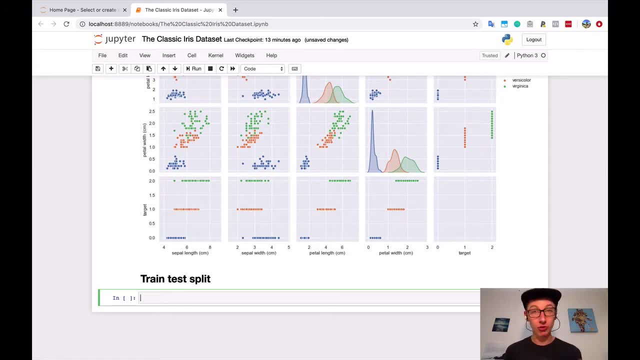 There's also going to be something that we do in the middle, called cross-validation, which helps us during the training process. But this is, we're taking a piece of data and we're setting it aside for the very, very end. So to do that, I'm going to add an import. 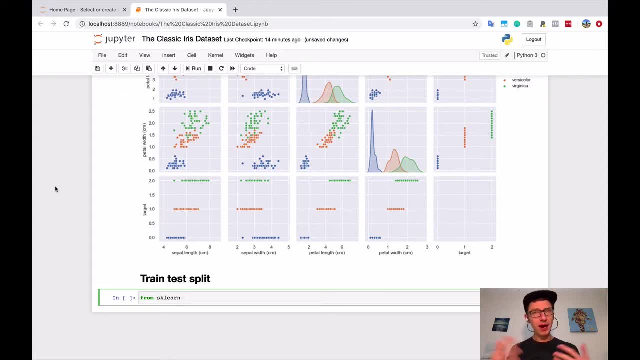 Down here, which usually in a Python script or in a notebook, I would put all my imports kind of at the very top. since we're just walking through this Linearly, you know kind of step by step here, I'll just put it down here for now. 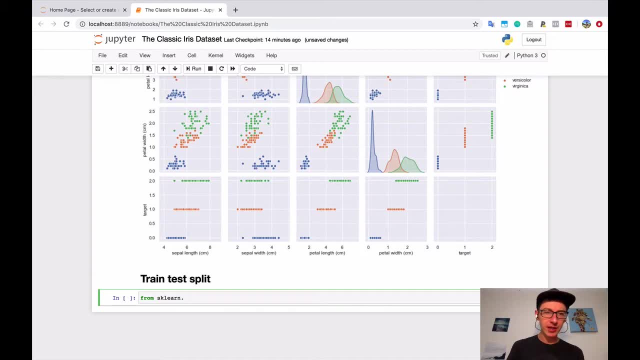 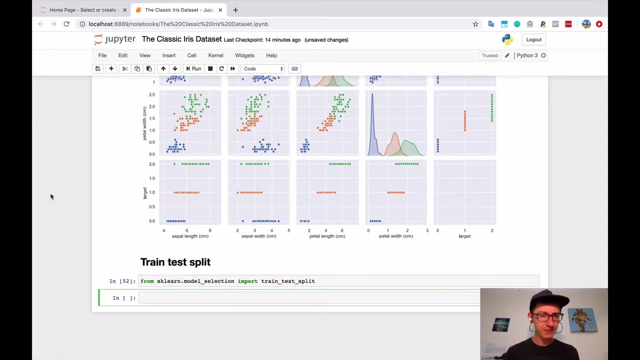 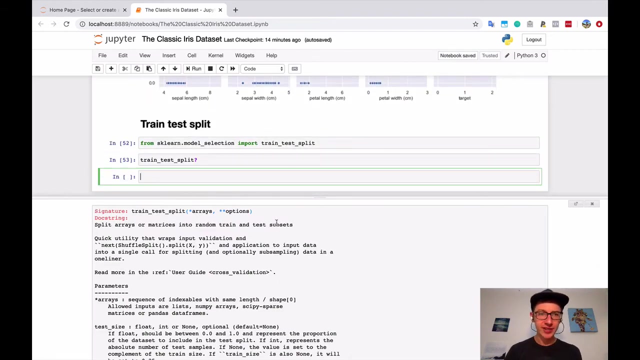 But from scikit-learn, from sklearnmodel-selection, let's import train-test-split And let's look at the documentation here. Okay, So splits arrays or matrices into random train and test subsets. So you pass in your arrays, You can pass in multiple arrays. 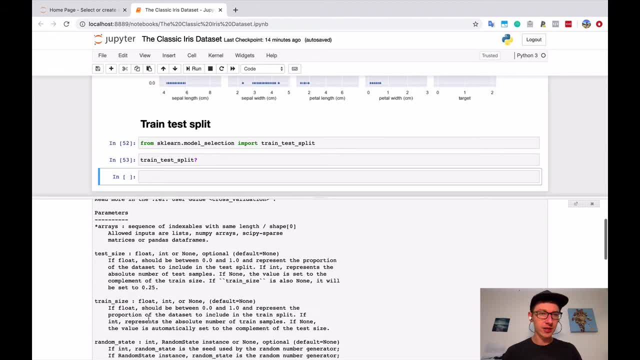 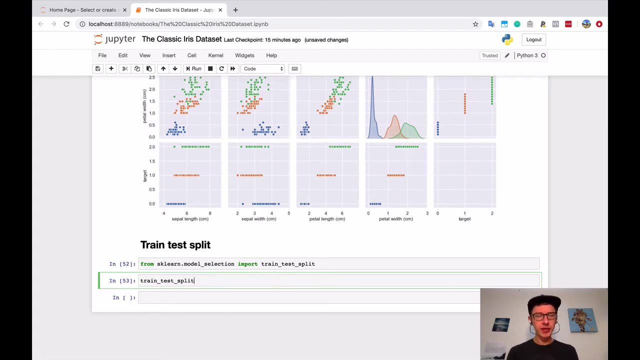 And then you pass in your options here, And the option that we're going to use is test-size, Test-size. So I believe it defaults to 0.25.. We'll just be explicit in passing that in, So train-test-split. 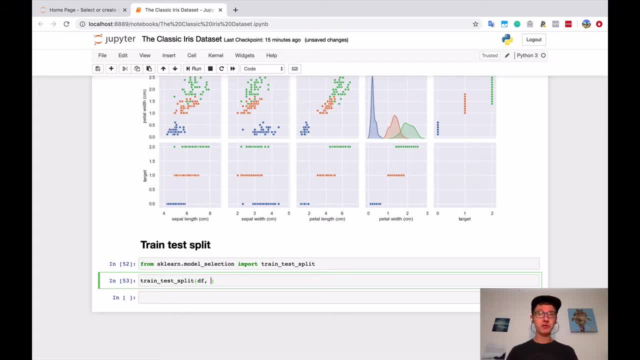 Let's pass in our data frame. So we're going to pass in our full data And let's say test-size equals 0.25.. And what this is going to give us is going to give us a train and a test data frame. 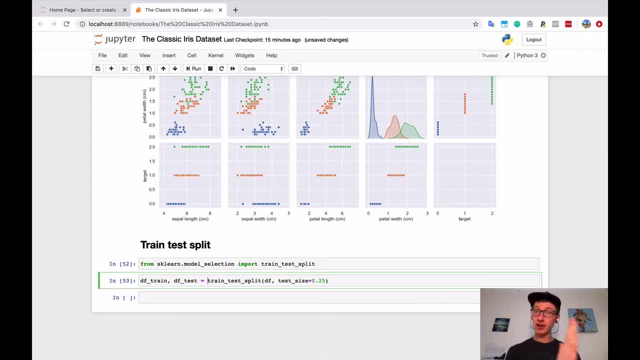 It's going to take our data that we pass in, split it up into 75% of our data which we're going to use to train on, and then 25% of our data which we're going to forget about until the very, very end. 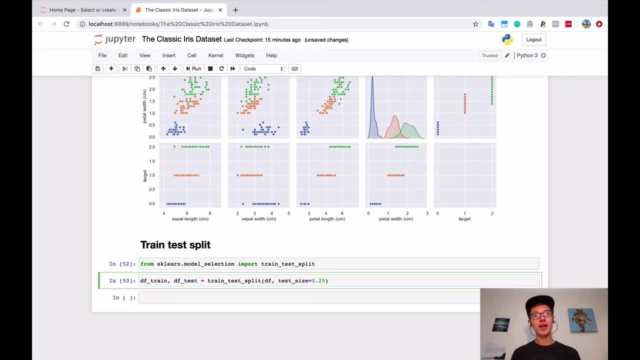 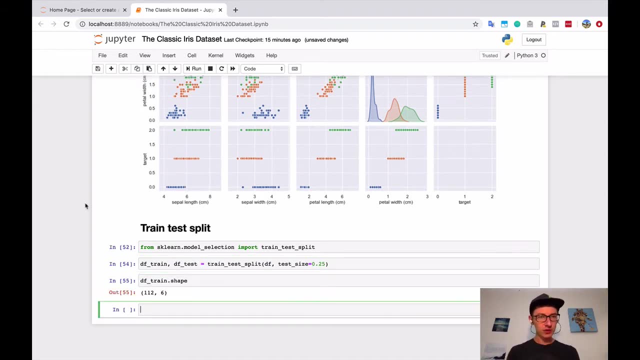 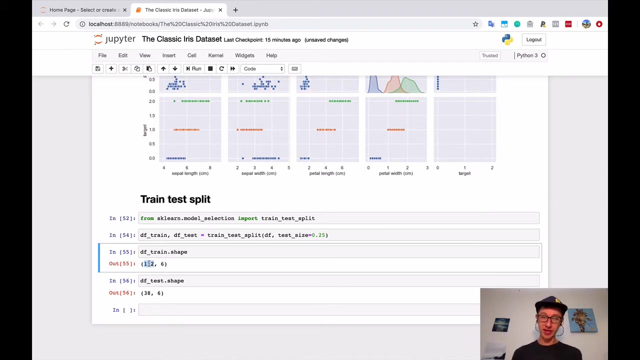 And then we're going to use that to evaluate our final model. So let's go ahead and run this And let's just look at these shapes here, So you'll notice that we have 112 rows of data for our training data and 38 rows for our test data. 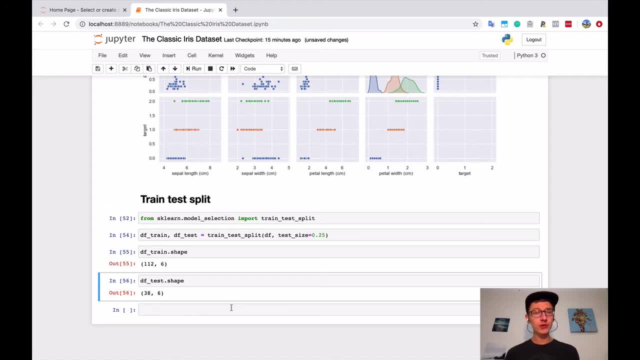 This is a very small data set, So you always want to have as much data as possible- Okay, As much training data- as you possibly can. This is pretty small, So we could even reduce the size of our test set if we wanted to. 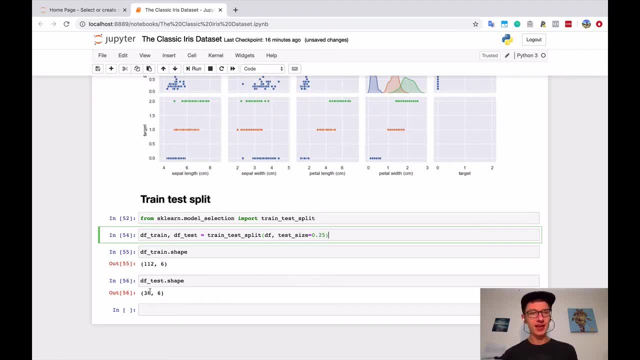 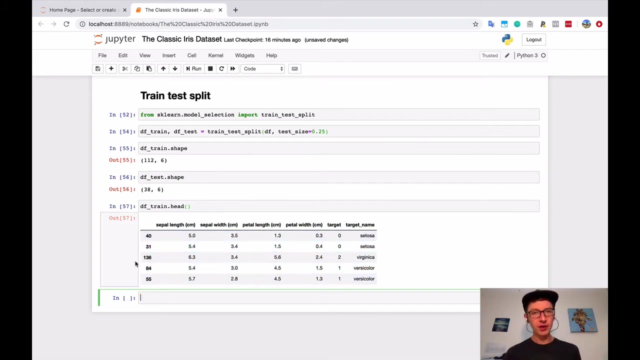 But we'll leave it as 25% for right now. And these add up to the full 150 data points that we started with. And if we look at dftrainhead, you'll notice that the index is shuffled first of all. 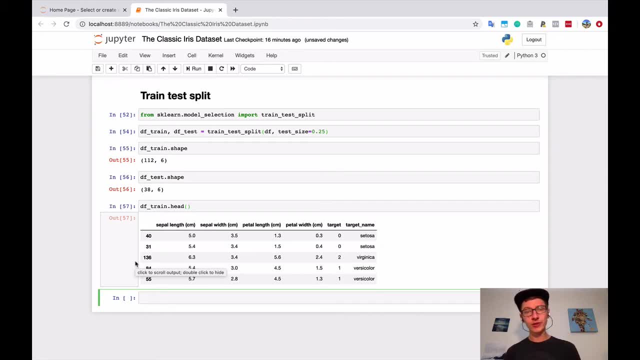 Train-test-split shakes up our data For us And that we've still got our four features, our target and then, just for our reference, our target name as well. So now that we've done this, let's go ahead and prepare our data for modeling. 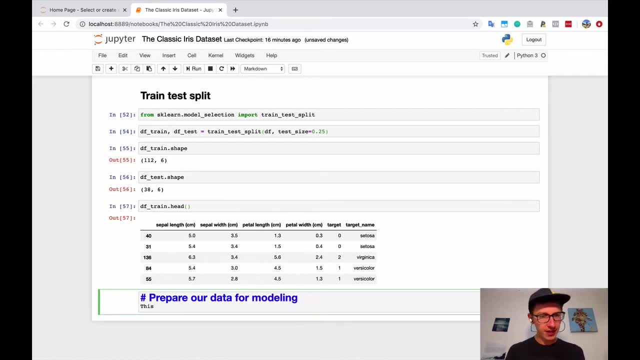 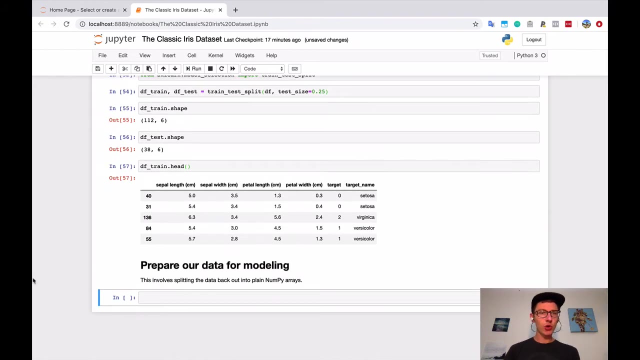 And we're going to say this involves splitting the data back out into two, Back out into plain numpy arrays, And so this is partially why we could do this whole process just using numpy as well is because scikit-learn takes numpy objects and uses those to do the modeling, to do the machine learning. 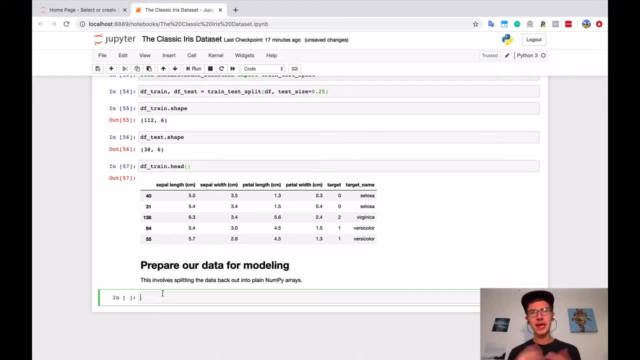 So we could have just stuck with numpy the whole time. But pandas does provide some nice functionality And it's easy enough to split it back out. So we're going to have our X training data, our Y training data. So this is going to be this dftrain. 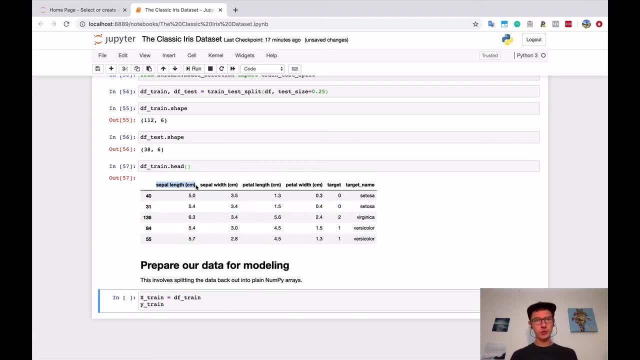 And rather than saying what columns we do want, we can approach this a different way. We can say what columns we don't want by dropping them. So we'll drop this, So we'll drop the columns target And we'll drop the column target name. 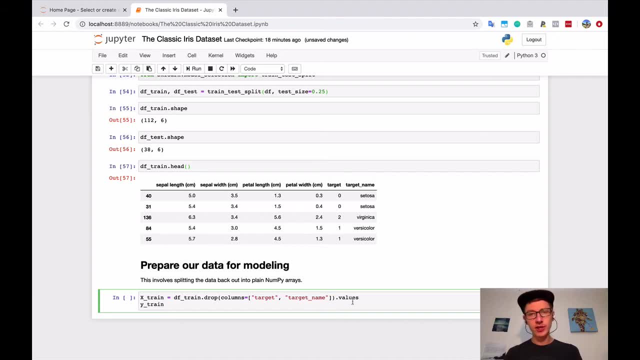 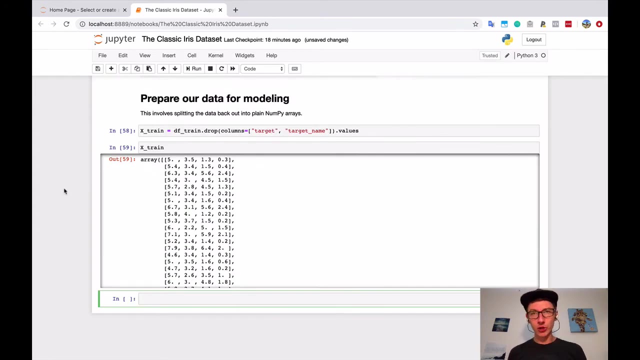 And then we'll use the dot values attribute to. So we're going to drop those columns first And then we're going to get the values, which is the numpy array version, And we'll just run this really quickly And I'll show you that on the output side we get something that looks very similar to what we originally passed in. 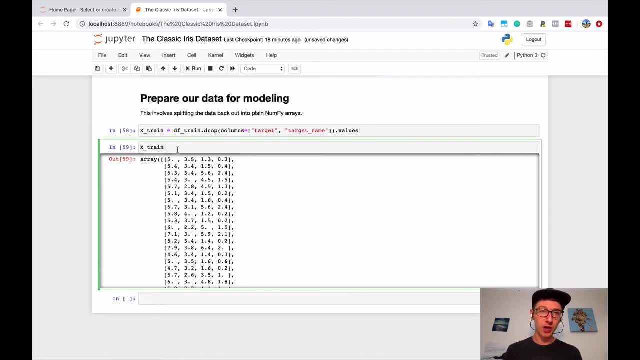 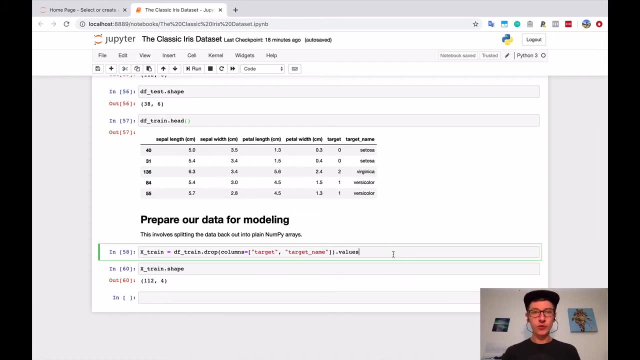 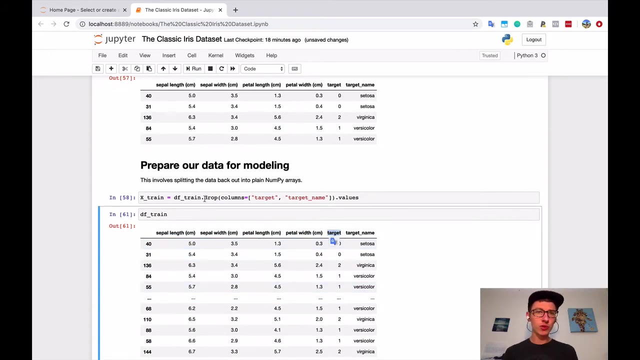 Which is a numpy array with four columns and 112 rows. So, and then, if you look at dftrain, those columns that we dropped are still going to be there, Because this, whenever we say dftraindrop, this returns a new object. 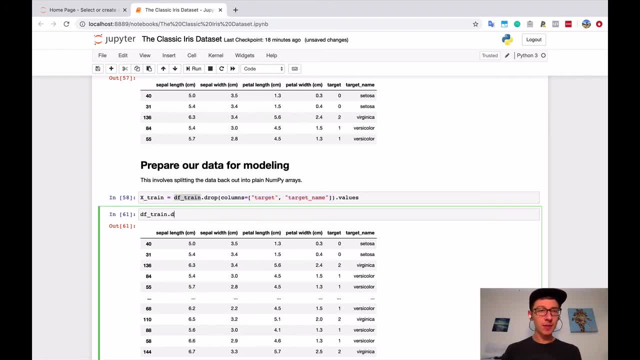 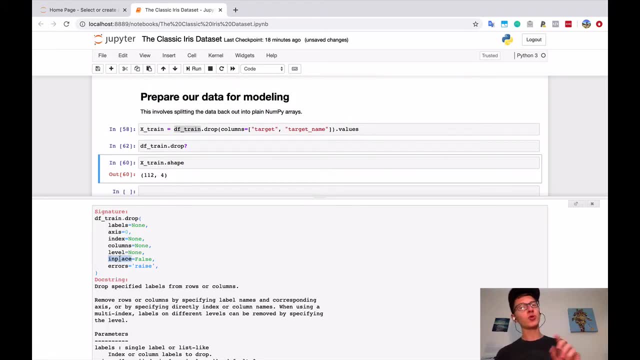 And it doesn't change this object, Unless we were to say this function has this parameter called inplace, And you'll see this with a lot of pandas functionality, Where inplace is a parameter that you can pass in to a data frame, And usually it's false. 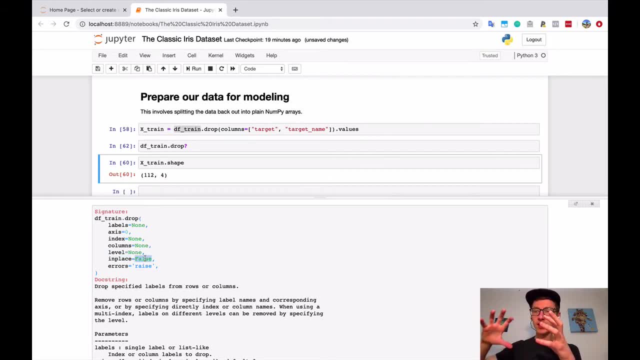 Which means that pandas is going to take your data frame. It's going to create a copy of it, Create a new version, Make all your modifications On that And then give you that new version back, Leaving the old version unchanged. Now, if we wanted to actually drop those columns. 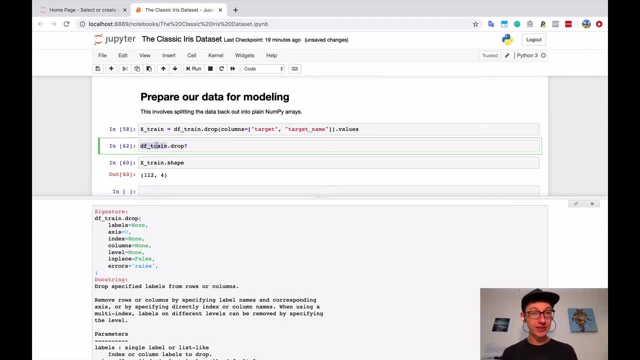 And we wanted to do it on this original data. Then we could say: you know, inplace equals true, And that would alter the original object. And this is something you can play around with, Definitely. you know, if you're new to pandas, play around with it. 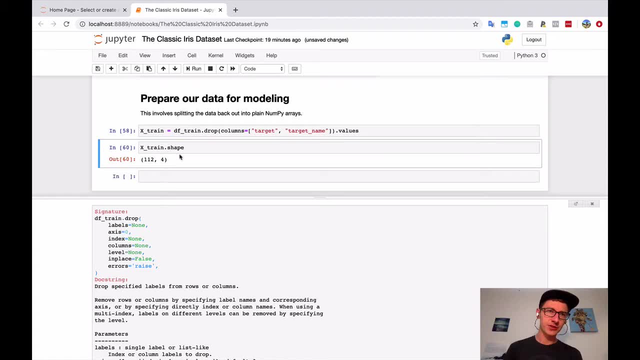 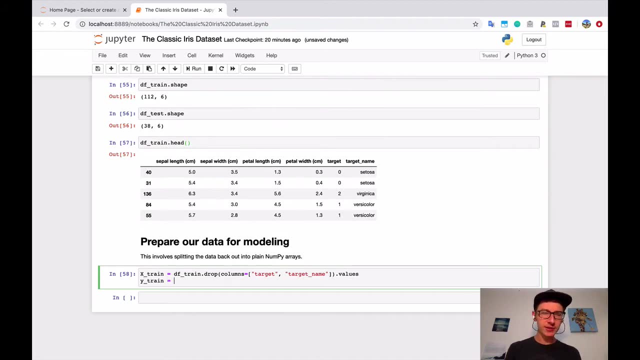 Get a feel for it. It's definitely a good thing to do there And in this cell. let's go ahead and create our Y train data as well, And in this case, that's just going to be the target, Which is what we started with. 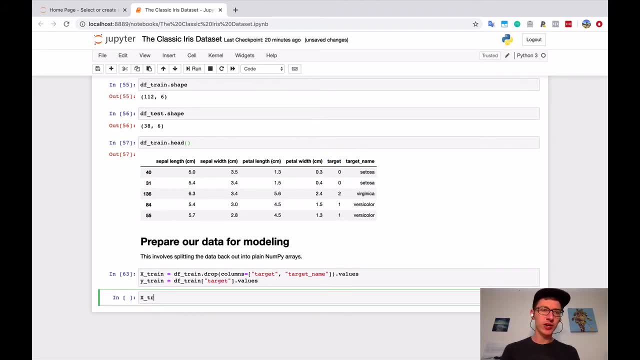 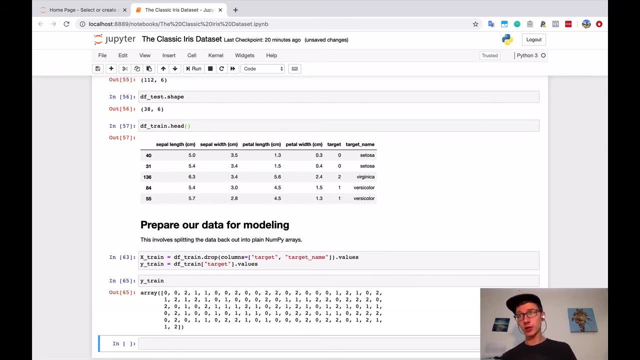 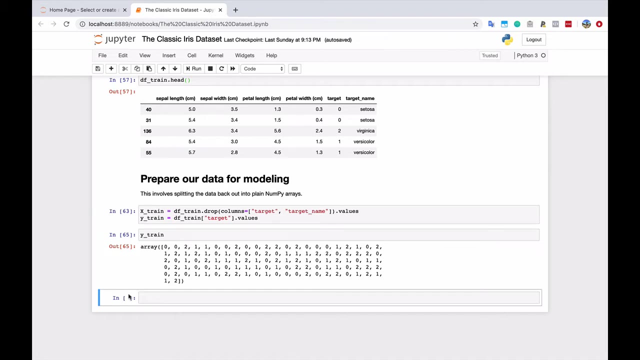 If you remember. So we look at our X train data- That looks good. We look at our Y train data- That's looking good. All right, Okay, So we have our data ready for modeling now. So, before we pick a specific model that we're going to use, 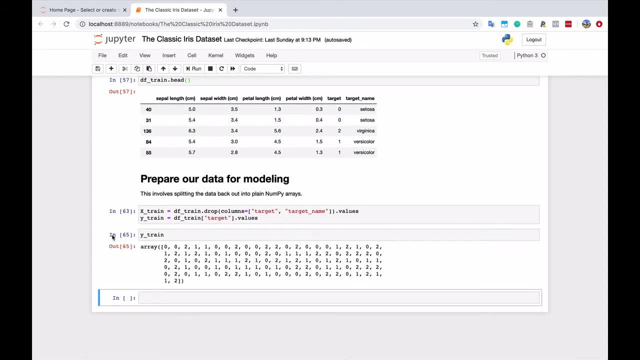 We're going to use logistic regression in this mini course here, But before we do that, one of the things that I like to do- And I think that is a best practice- Is just ask the question: what is our baseline? And so by baseline here what I mean is the simplest model. 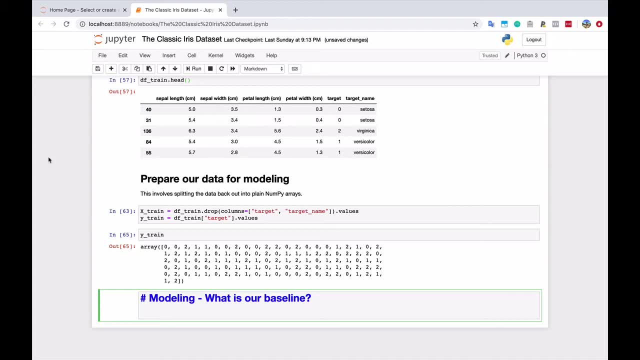 That you could create, So something that's- you know that's not intelligent in any sense- Like random guessing essentially. So like if we were just randomly guessing the answer here, What kind of results would we expect to get? So I'll go ahead and write that down here. 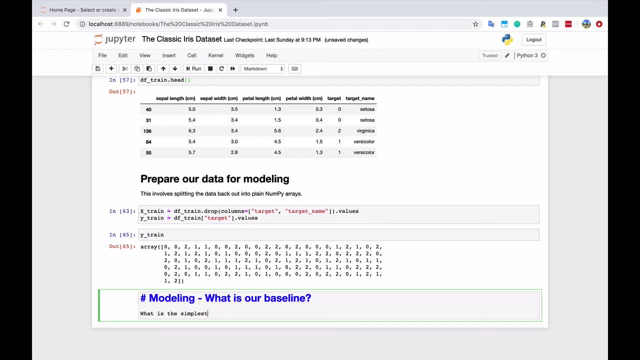 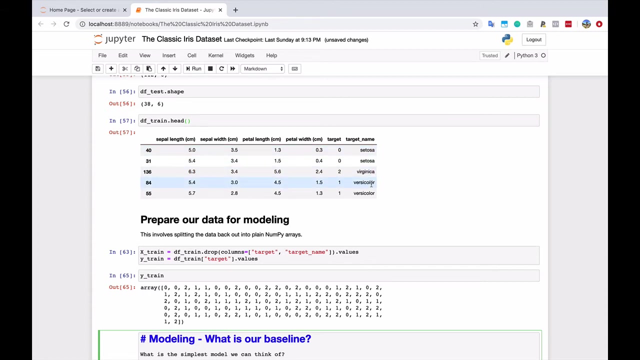 So what is the simplest model we can think of In this case? if our baseline model is just randomly guessing the species of flower, Then we would expect to get the answer right. So we have 50 different data points for three different classes here. 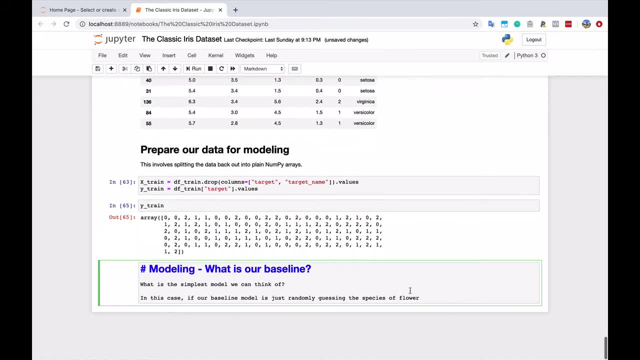 So 150 data points total. So if we're just randomly guessing what flower species it is, Not using any of our X-train input data, We would expect to get the answer right. a third of the time, You know, we randomly guess setosa. 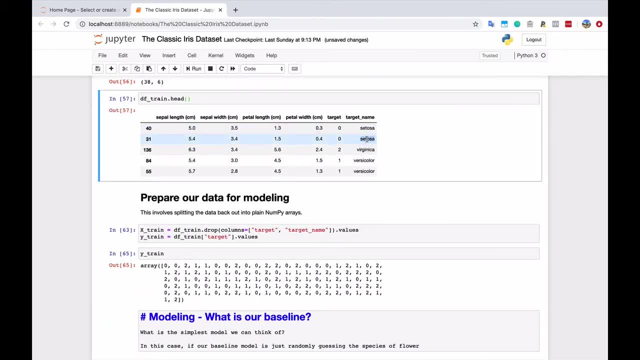 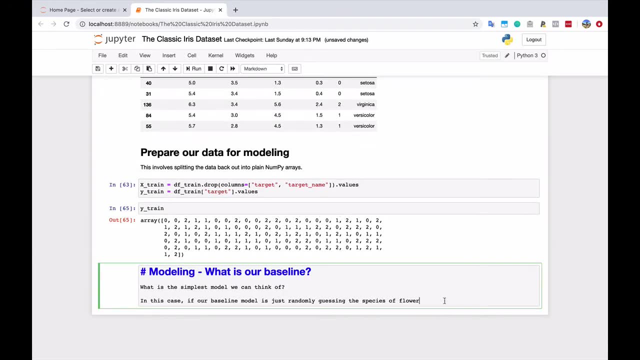 Or, you know, we could even just guess one of these class labels 100% of the time And still get 33% accuracy. Those are basically equivalent. So if our baseline model is just randomly guessing the species of a flower, Or guessing a single species for every data point, 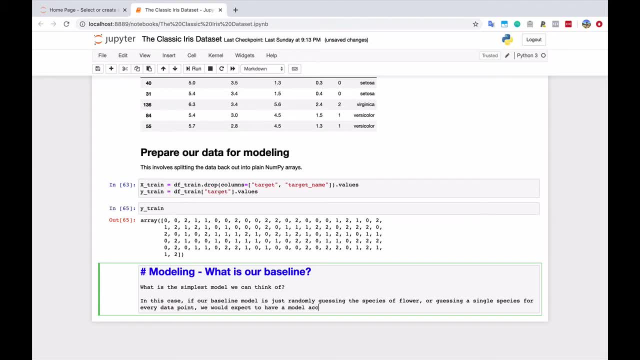 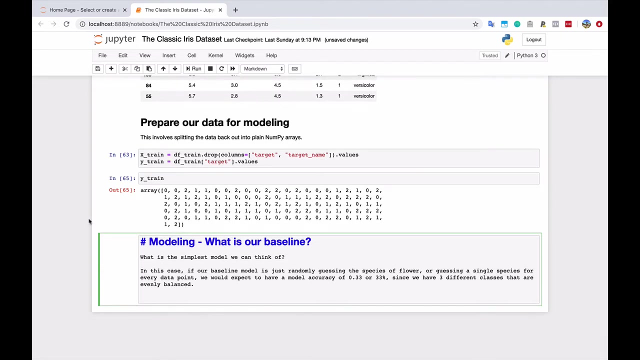 We would expect to have a model accuracy of 0.33 or 33%, Since we have three different classes that are evenly balanced. So 50 data points at least. So this is the absolute worst that any model we create should do, If our model isn't at least doing 33% accuracy. 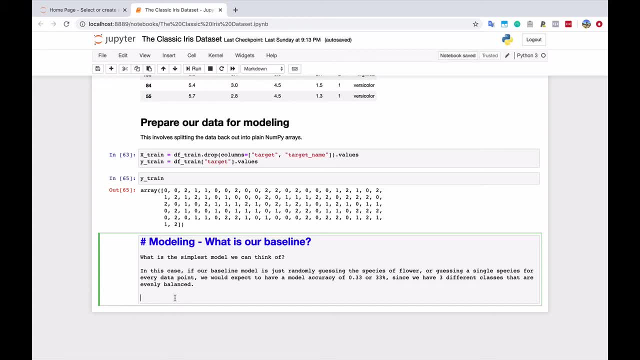 Then we would be better off by randomly guessing. So this is kind of the floor, And this is a good thing to do for any model that you create, Because a lot of the time, especially if your classes are imbalanced, You know, let's say that 99.. 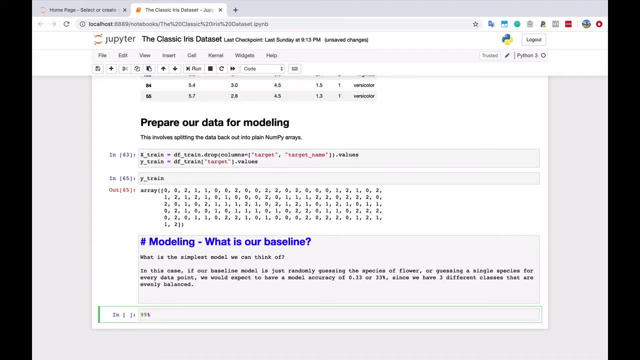 You know, if you've got like 99% of your classes, Like 99% of your data points all belong to one class, Like, let's say, 99% of our data points were setosa And only 1% were virginica. 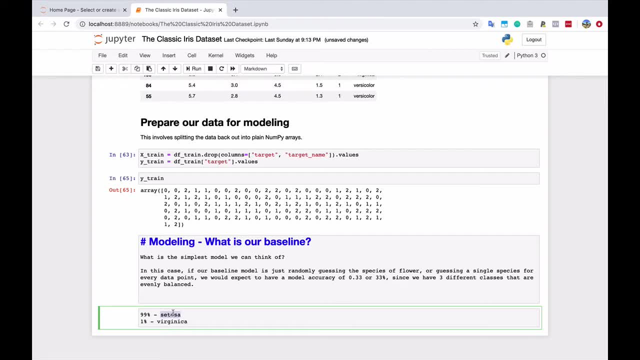 Well then, guessing setosa for every single flower would give us a 99% accuracy, But we wouldn't really be modeling anything there. So this kind of baseline question is really good to ask Anytime that you're doing any kind of modeling. 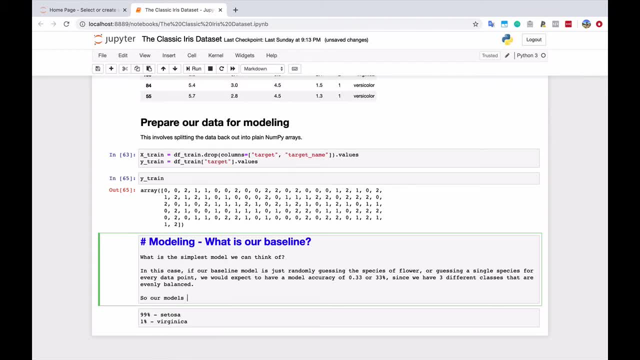 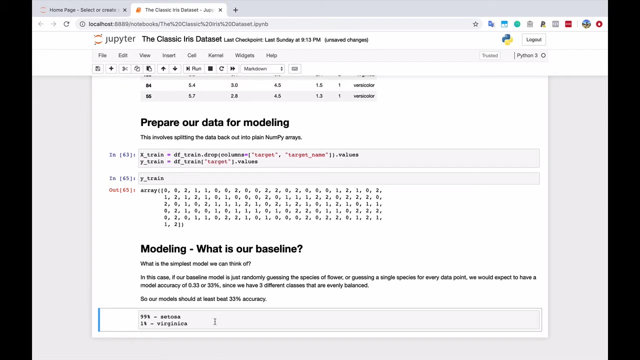 So our models should at least beat 33% accuracy And, as you're going to see, we're actually going to do much better than that. So let's actually take this one step further Before we get to. you know what we might normally think of as a statistical model. 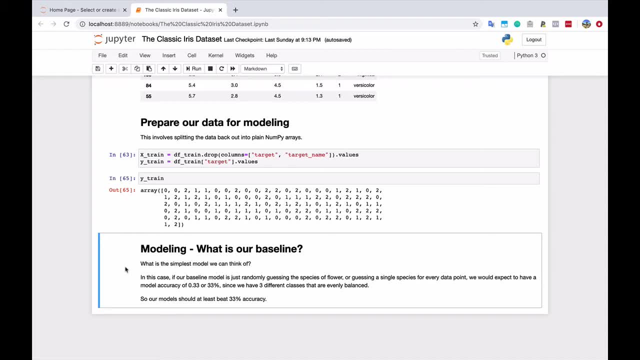 Or a machine learning model. I want to show you that modeling at its most basic sense, you know, fundamentally Is just about mapping inputs to outputs in an intelligent way, And that doesn't require any kind of fancy equations. So let's do a, we'll do a simple. 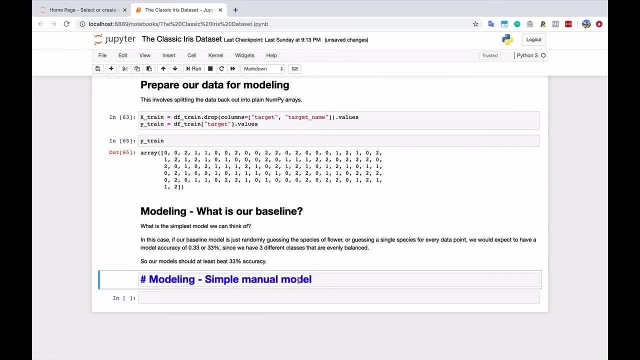 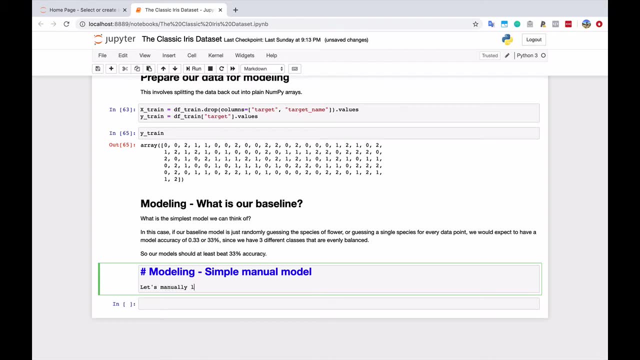 We're going to do a simple manual model to start with. And so what do I mean by that? What I mean by that is Let's, Let's manually look at our data And decide some cutoff points for classification, And you know, all of modeling is going to be essentially doing the same thing. 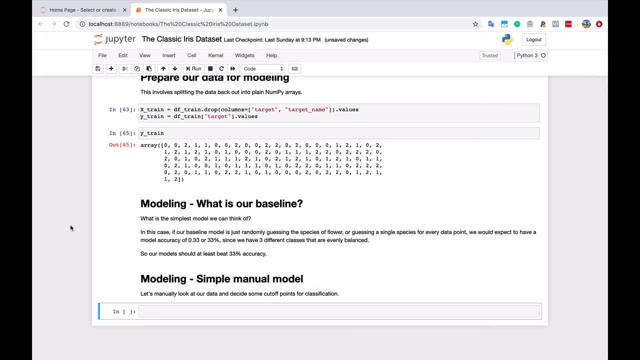 Just in more or less you know complex ways, With various reasons for doing things differently, But at its basic, you're just deciding how to map input points To an output that you care about modeling. So let's go back up to our graphs here really quickly. 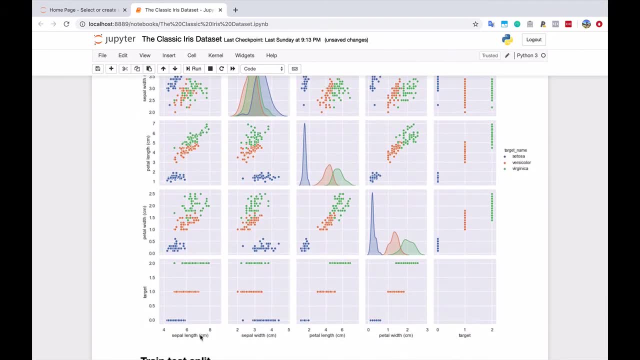 And let's just take a look at our input data. So remember that our input data is sepal length, sepal width, petal length, petal width And our output that we want to model is the flower species here, So setosa, versicolor and virginica. 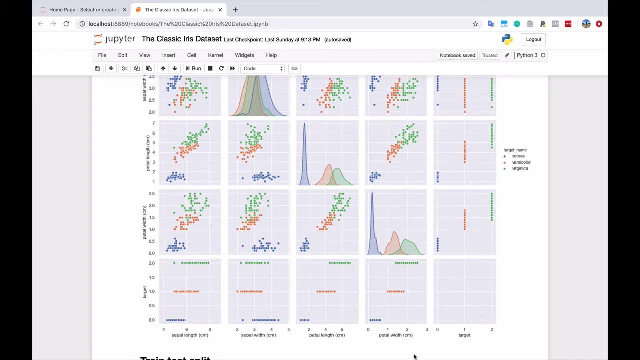 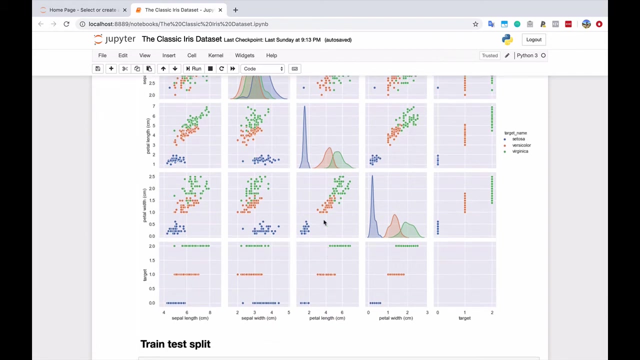 And we want to use these four input columns, These four input features, to model our output. Which is this category, This categorical, you know, classification, essentially. So if we were to do this manually, How would we do this? So let's take a look here. 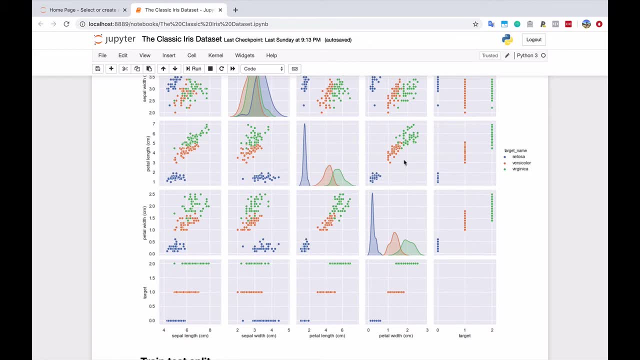 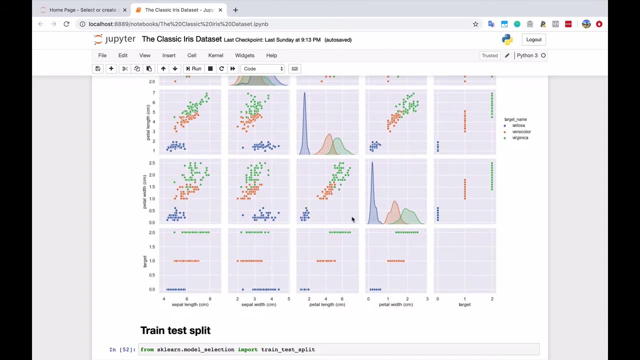 It's easiest to start with setosa. So setosa, you can see, is really nicely clustered Apart from the other two species. So this plot right here actually shows this very nicely. So this plot, which is what is this? 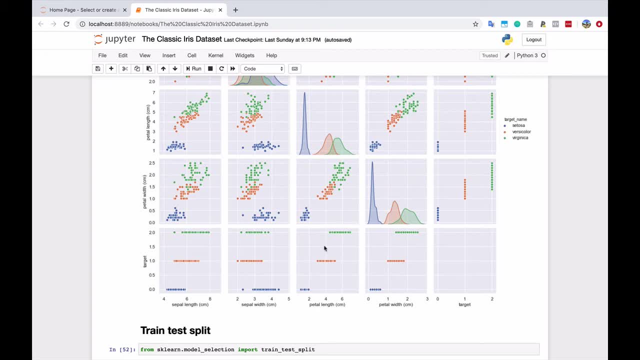 Petal length along the x-axis here Going from like one centimeter up to, you know, seven or eight centimeters, And then versus petal width, Which goes from you know like 0.1 centimeters all the way up to 2.5.. 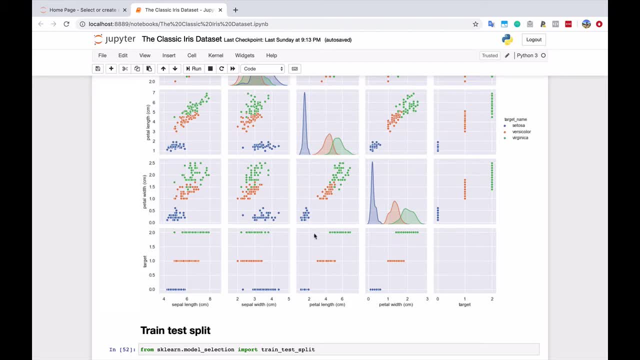 And if we were to segment This off, If we were to kind of decide some classification rules here To segment off setosa by itself, What would we pick? Well, if the petal length is less than, what is this less than? 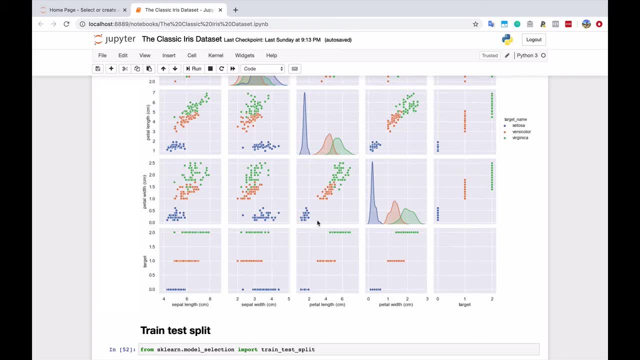 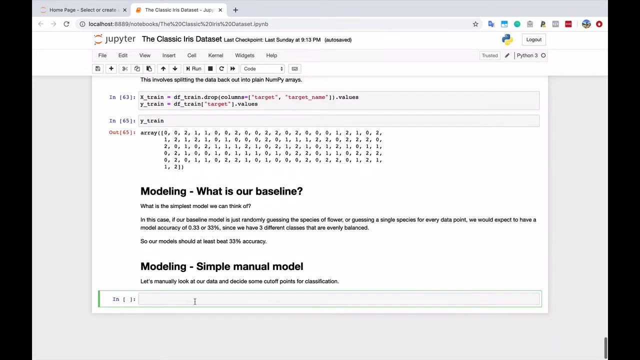 Like 2.5. So like this is three right here kind of in the middle, So 2.5. So if petal length is less than 2.5. Then that is clearly indicative of the setosa species. So actually that can go ahead and be our first classification rule. 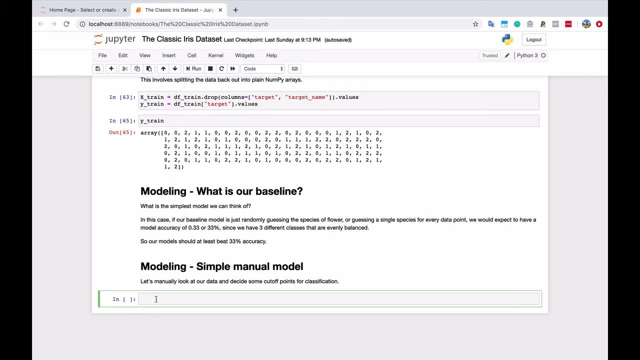 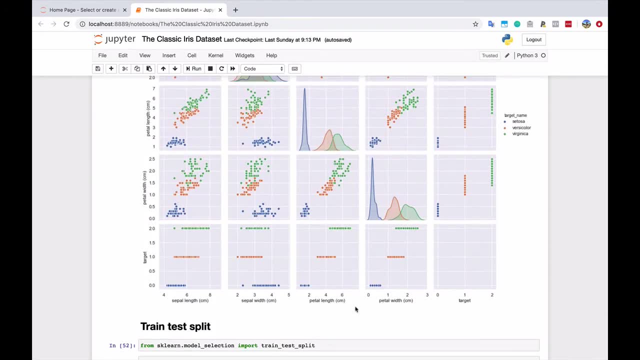 So how do we do this here? Well, maybe, let's, maybe let's just make our classification off of this one feature. So we'll just stick with using one feature And we will classify all three of these species based on just this one input. 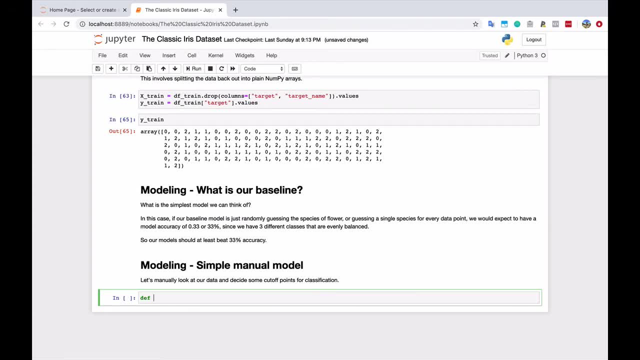 So maybe I'll create a function And I'll call this function single feature prediction, And we're going to pass it a petal length And I'll give it a very simple doc string here Which is: predicts the iris species given the petal, the petal length. 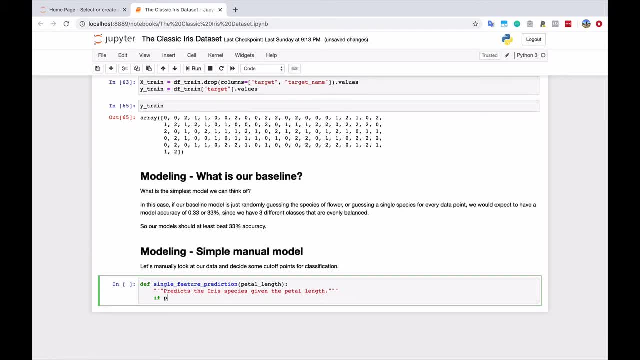 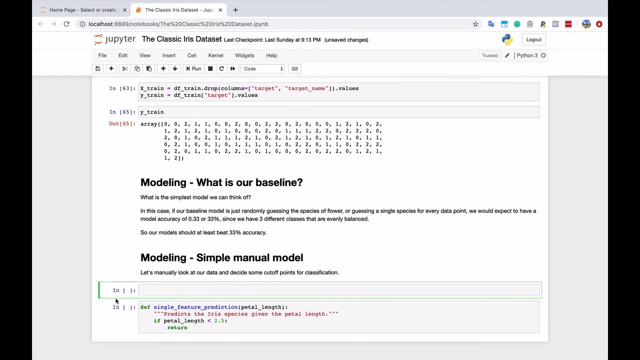 So our first classification rule here would be: You know, Petal length is less than What? did we say 2.5.. Then we're going to return. Well, we could return setosa, But let's, let's return maybe the, the number instead. 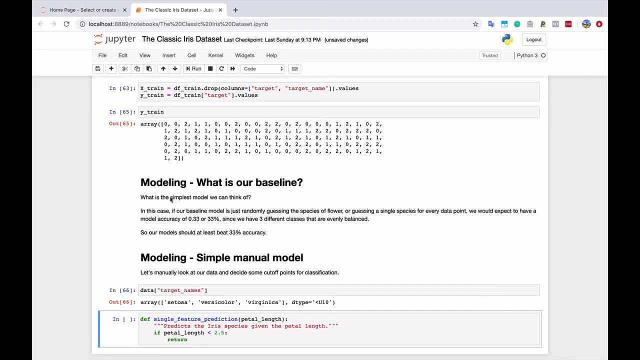 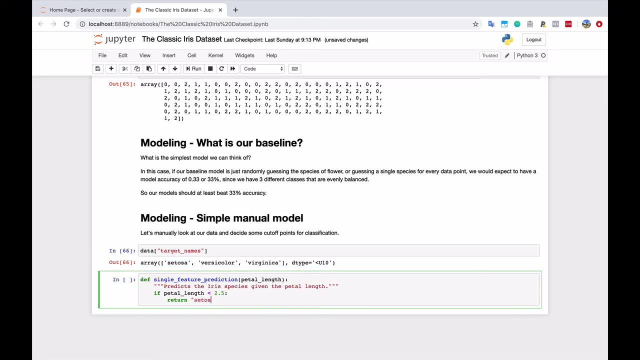 So if we look at our target names, Looks like setosa is index 0 here, So we could either return- you know, setosa, Or in my case, I'm just going to return 0. To indicate that this is the 0th index there. 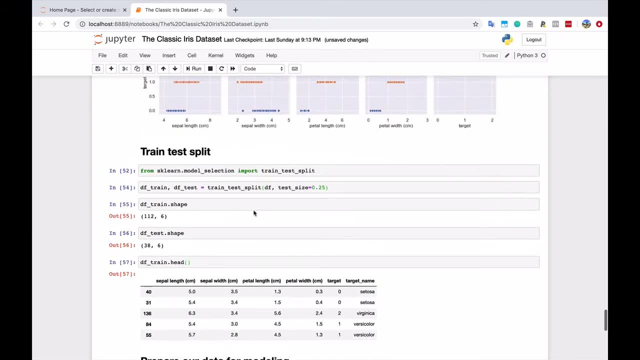 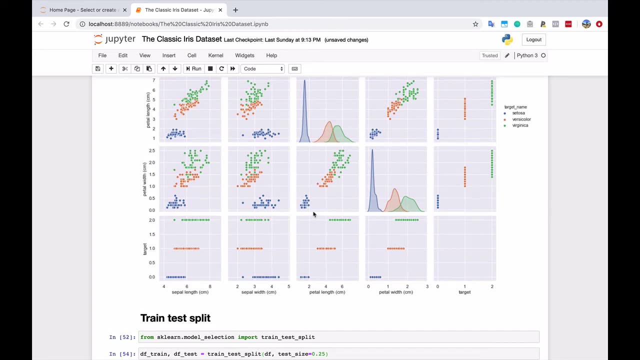 All right, Let's go back up to our graph Now. So let's say that we've already segmented this off, You know? So if, If petal length is less than 2.5.. Then we classify it as setosa. 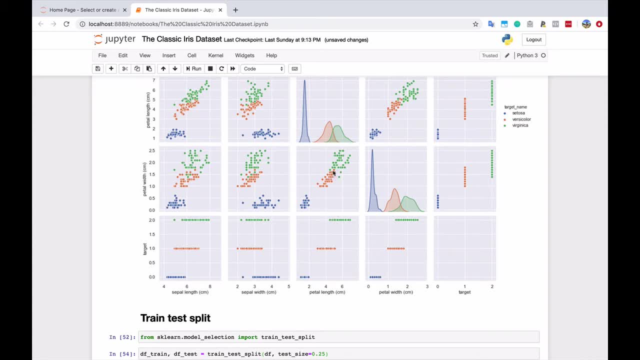 Well, now, How do we classify these other two? Now, this is where The cutoff gets a little messy, right, And this is usually how data science problems are going to look: Where there's There's not A clear dividing line. 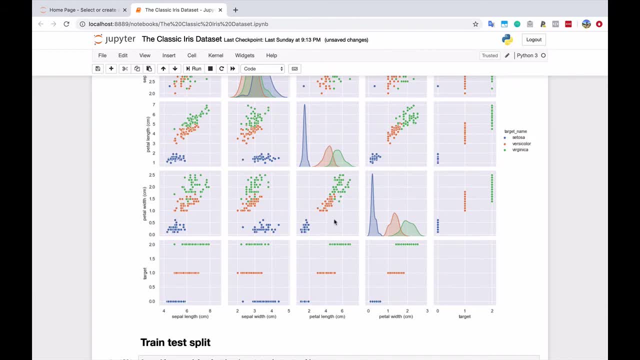 Between The different things that you're trying to predict. That's why it's a hard problem And that's why usually We want to use all of the information that we have. So we'd want to use all four of these input features. 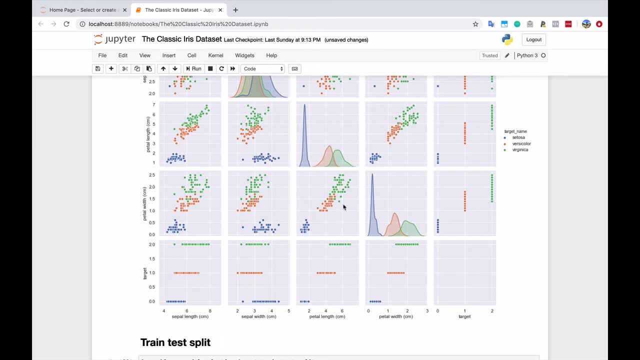 To get the maximum amount of information In order to make this classification, But for now, Since we're doing this manually, We're just going to use this one. So What is this? Let's see This cutoff Right about here. 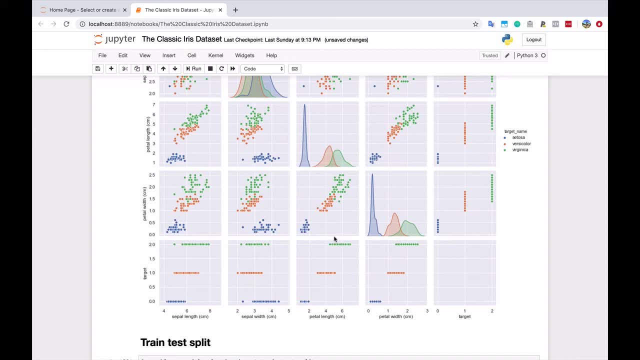 It's somewhere Just below five, So maybe not quite five, Maybe like Not 4.5. Maybe like 4.75. Or 4.8.. What if we go with 4.8?? So We'll say: 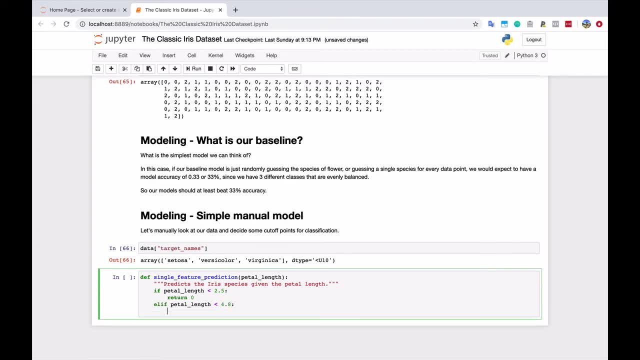 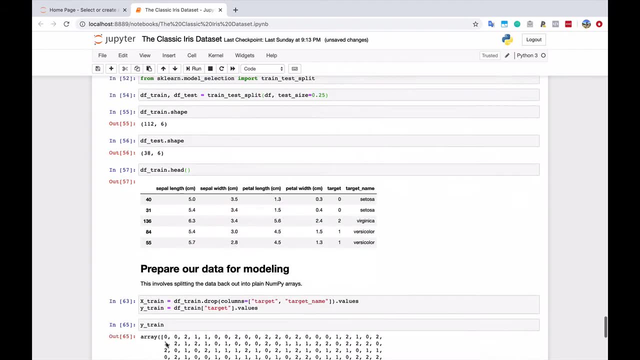 Elif, Petal length Is less than 4.8.. Well then, we're going to classify this as What? What species is this Orange? That's versa color, Which is Index one, So we'll return one. 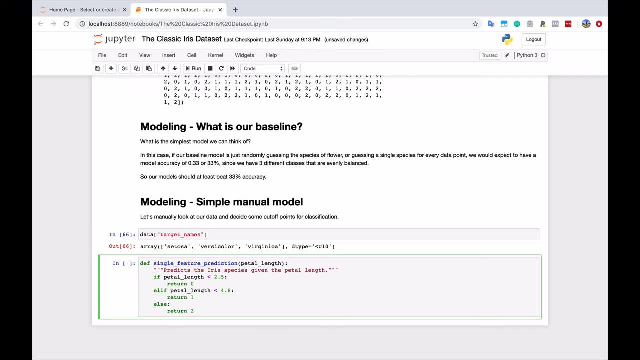 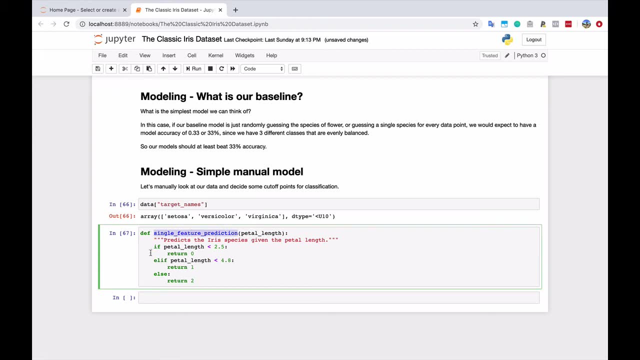 And otherwise Then we classify it as virginica And we return two. And so This Is basically our model, This single, This single function here with With very simple, You know If else rules, And You might be surprised to learn that this is actually. 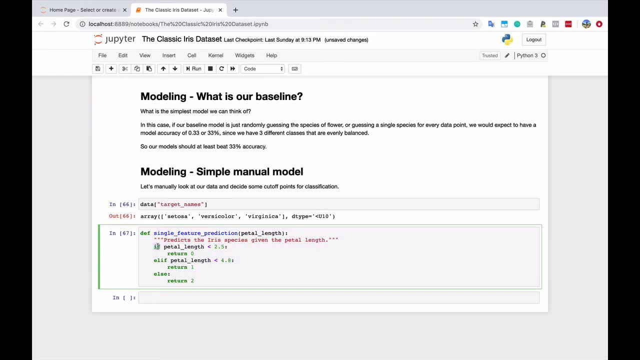 Kind of what happens for some machine learning models. So there's actually A tree based model, So decision tree Based models Which do Basically This Kind of If else thing. They just They automatically do it for you. 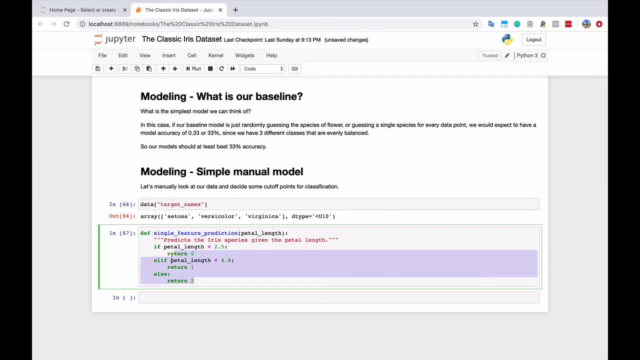 But under the hood, You know You're just doing a bunch of if else statements, And that's what decision trees are, Which are, Or You know They used to be very, very popular Machine learning models. I think that 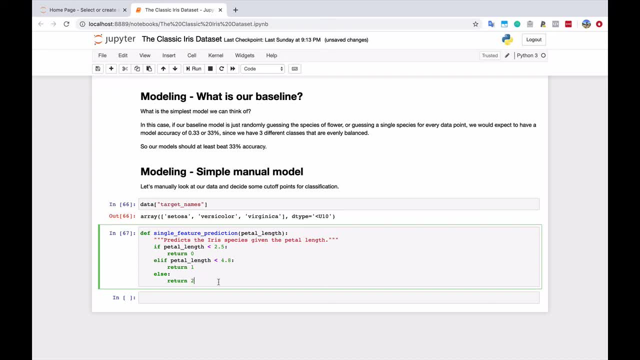 Maybe these days Not quite as much anymore, But You'll still see People using tree based methods Like random forests And whatnot So, So, So Let's take a look At Our. Let's see. 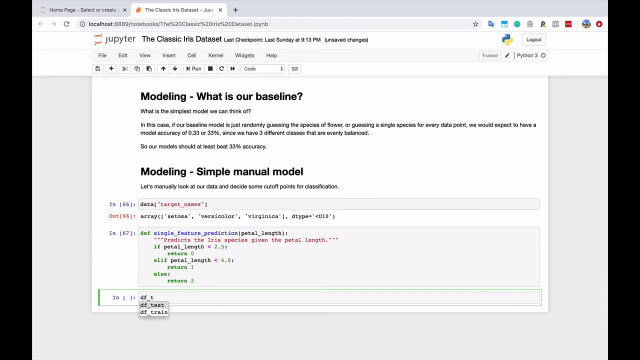 Let's take a look at our pedal length Values Here, And this is also going to be So if we use df train here. Let's see What Column is that. That's going to be the, The, The. 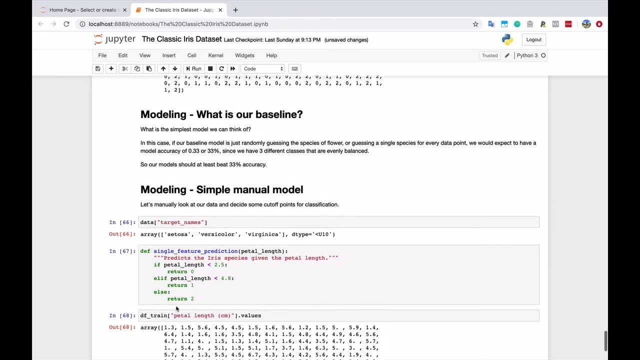 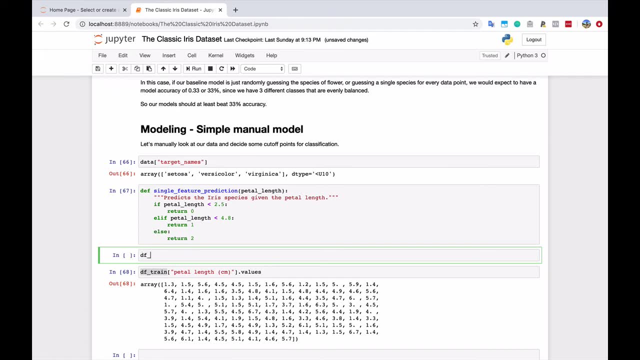 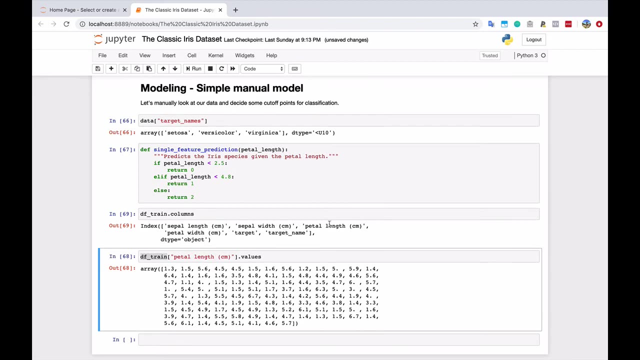 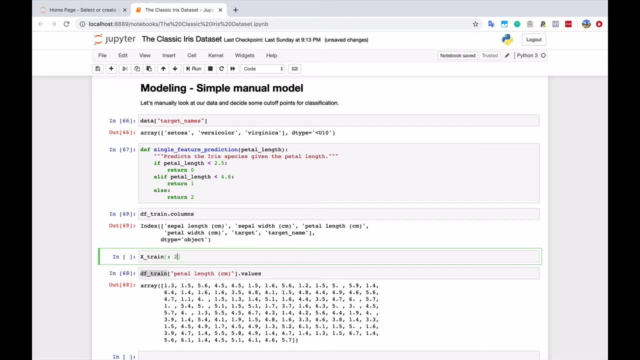 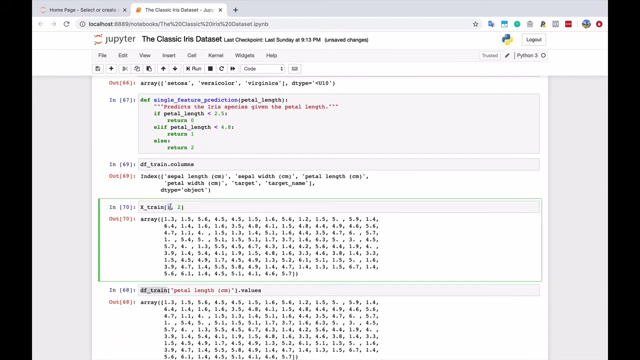 Here in our x Train And let's just make sure that those Are The Same. So We'll Do This Colon Here For All of the rows. Comma: The second Index Column. 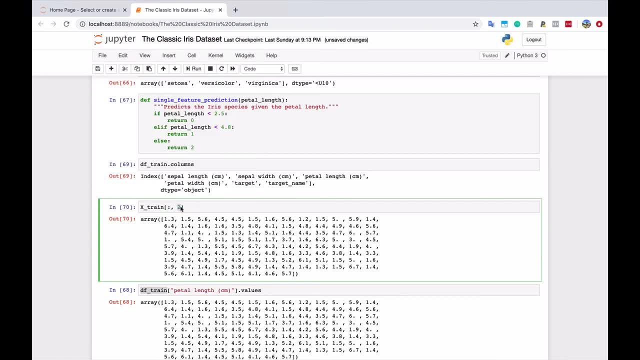 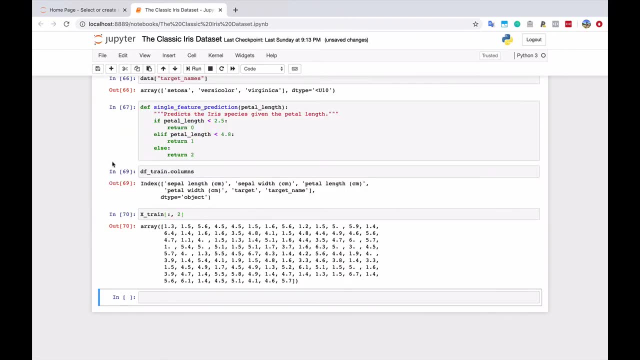 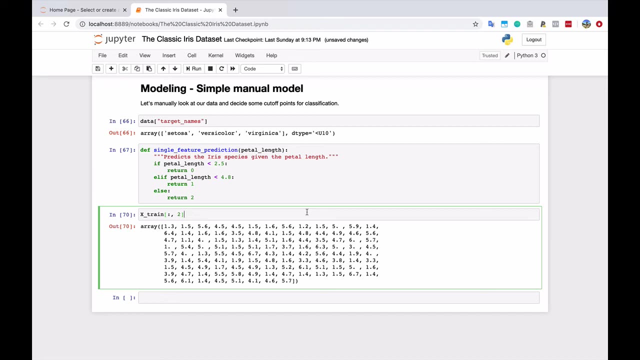 And that's. That's how you Specify things in one. after the comma is your column indexer. so, and that is correct, so I'll go ahead and delete this. we can use our X train. use our X train one. okay, so these are our petal length values. so if we wanted to make a prediction for each, 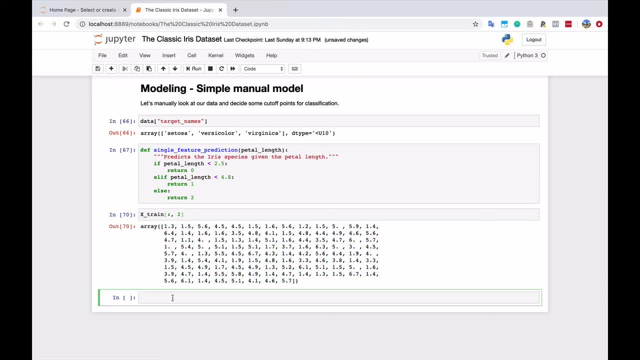 one of these. well, a simple way that we could think about doing that is we could do a Python list comprehension here and say single feature prediction. let's see: single, single feature prediction: Val for value for Val in X train colon for all of the rows and then two for the second indexed column there, which is petal. 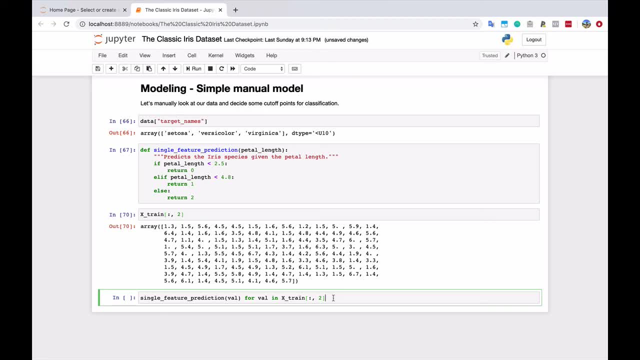 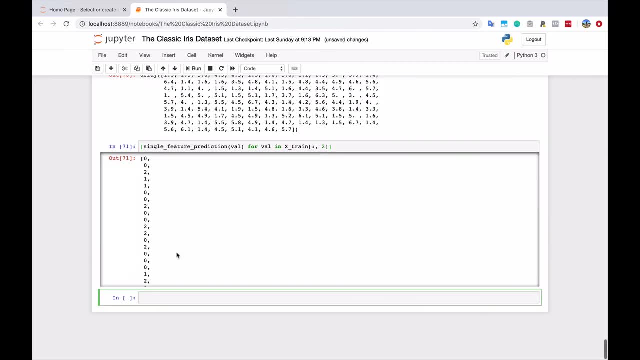 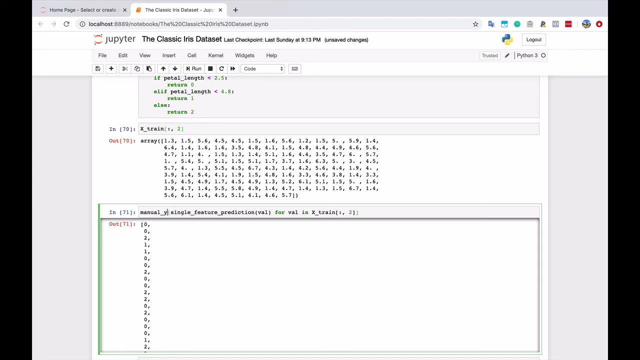 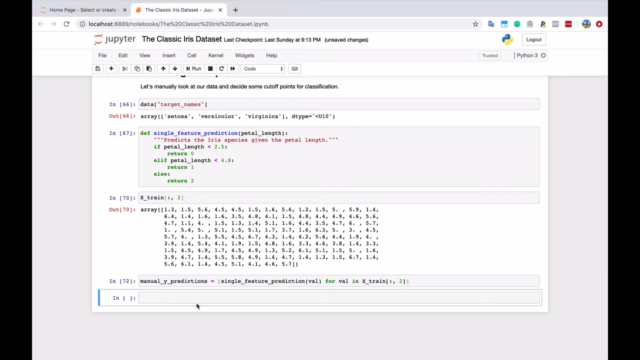 length and we do a list- comprehension- and this gives us a list of predictions that we make for all of the data. so let's, let's do this here. let's say manual Y predictions, all right. and so now maybe the question is: okay, how accurate were we? we're doing these predictions manually. 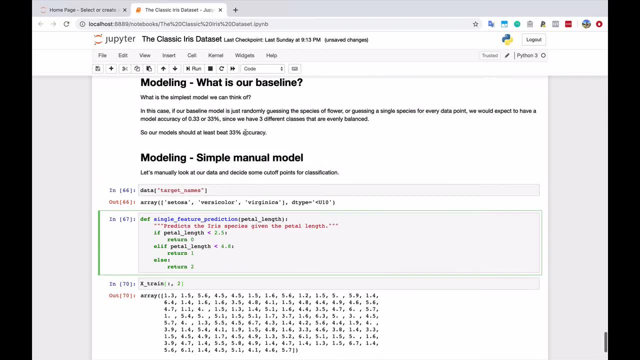 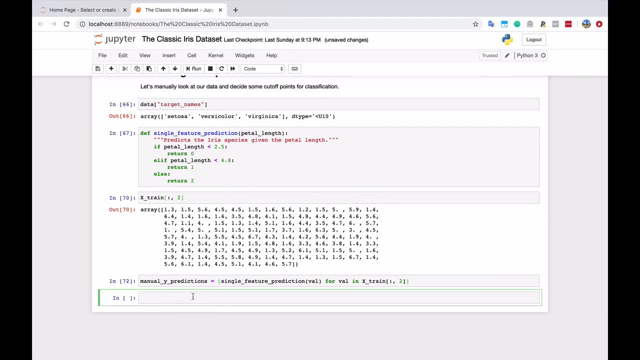 just using a single feature. so now, how accurate is our model? if our baseline model is 33% accurate, how accurate did we just get it? well, in this case, let's let's see here. so our Y train, that's our target. so these are the actual values. 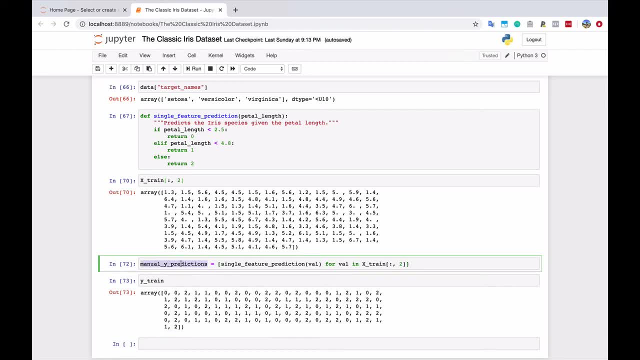 here, and then these, these manual Y predictions. these are the ones that we just created, and you know what? I'm gonna wrap this in NP dot array. I'm gonna make this a numpy array. let's just take a look at this, and I'm gonna go ahead and 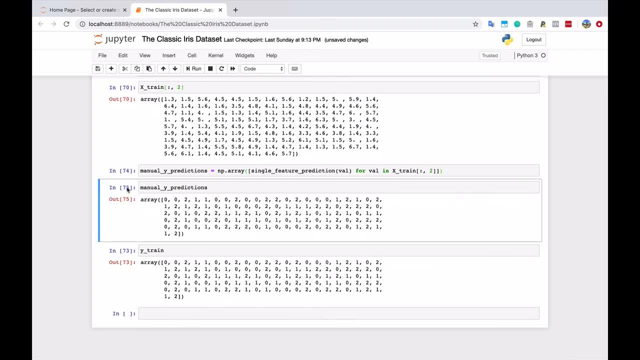 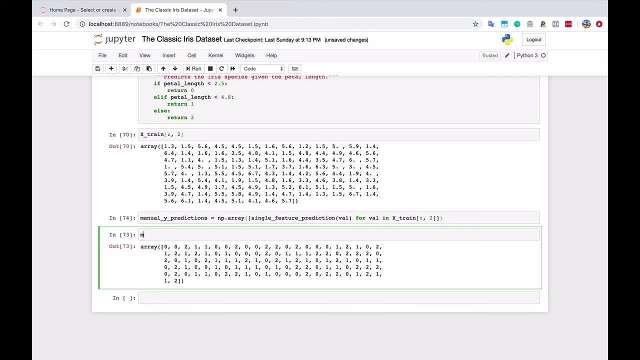 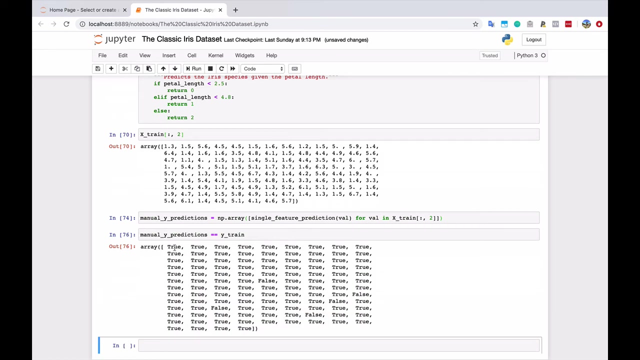 get that really quickly. there we go, and now it's just as easy as saying, okay, our manual predictions, we can set that equal to our Y train. so these are our true values for what species the flower is and this is going to create. we can do shift, enter here to run that. so this is going to be true every time that our 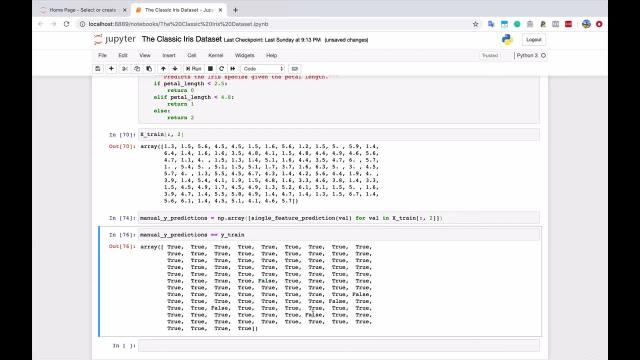 prediction is correct, and for that we're going to have to do a little bit of a false every time our prediction is not correct. and then a nice way to get the accuracy here is we can just wrap this with NP, dot mean. so it's gonna take the. 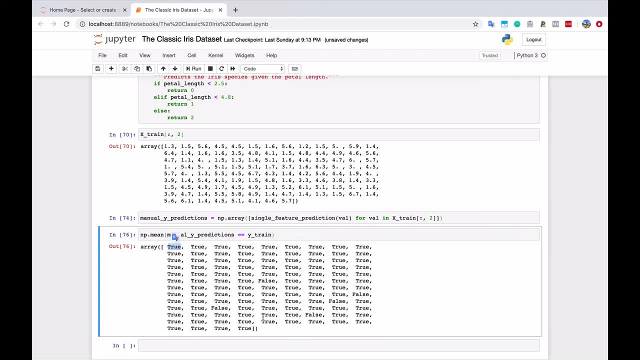 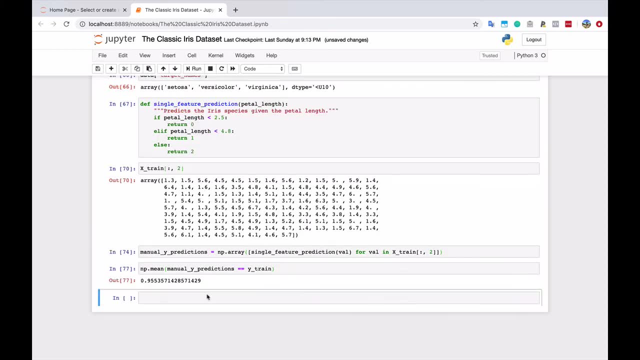 average of this. it treats all of the true values as ones, all of the false values as zeros. and then, by taking the average, we see essentially what percent of the values are true, and this looks like. ninety-five percent of the values are true, and this looks like ninety-five. 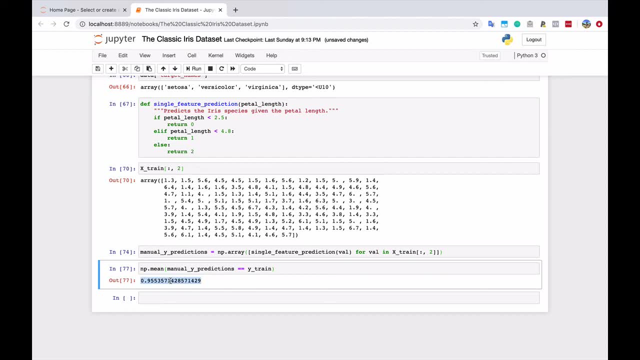 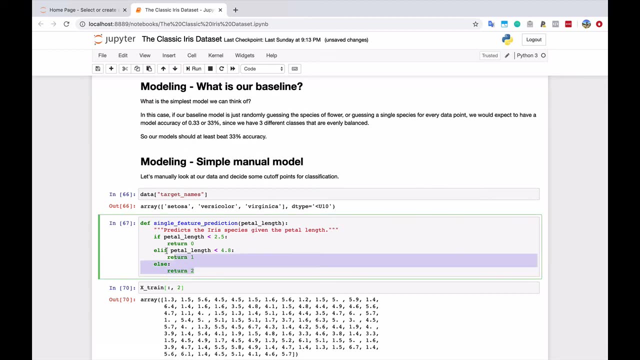 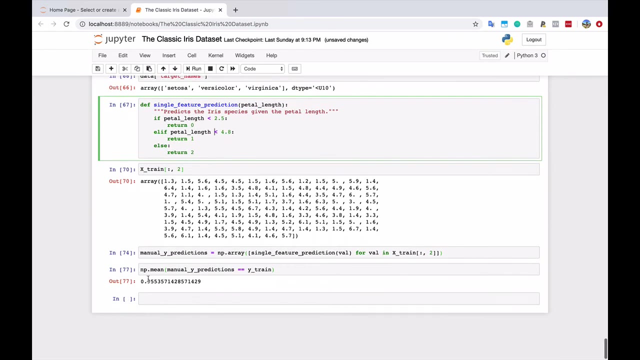 point five percent of the values were classified accurately. so that's pretty amazing if you think about it, if you think that we just defined this model manually, just using some if-else statements here, and we went from a 33% baseline accuracy up to ninety five point five percent accuracy. so this is: 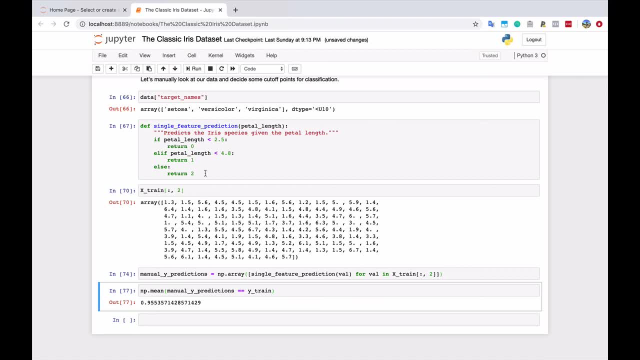 you know kind of fundamentally what modeling is doing, and it just so happens that this data set is a nice small, easy one to work with. but the reason why data science and machine learning are so interesting and why they're so important is because things are not always this easy and so 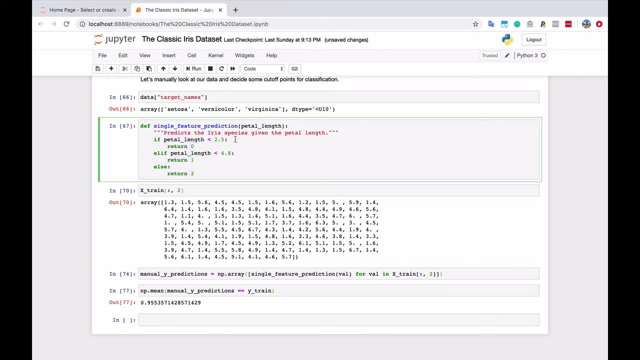 we need additional tools and techniques to help us whenever the problems get harder. so I'll go ahead and say that this is our manual model. accuracy equals that, and then, if we want to print it nicely, we can use an F string here and I'll show you what this does in just a sec. so manual model accuracy and then. 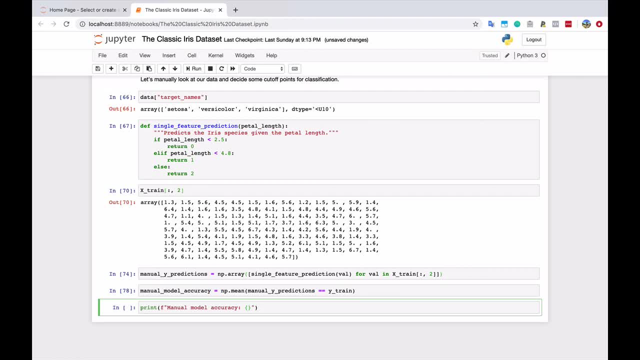 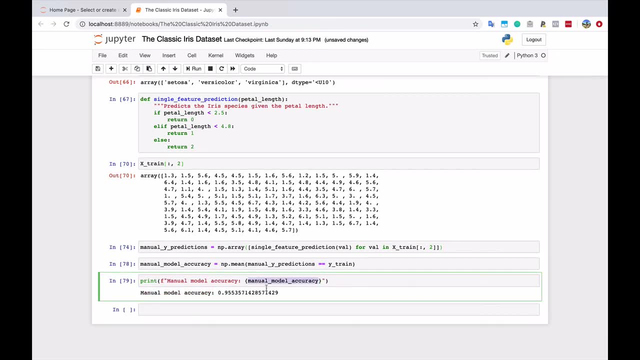 we can use the curly, the curly brace here, the curly bracket, to actually input our manual model accuracy and this is going to print this out with this string here. and then we can do some nice things here, like we can multiply this by 100 inside of the curly braces, so we can do normal kind of Python math in here. and 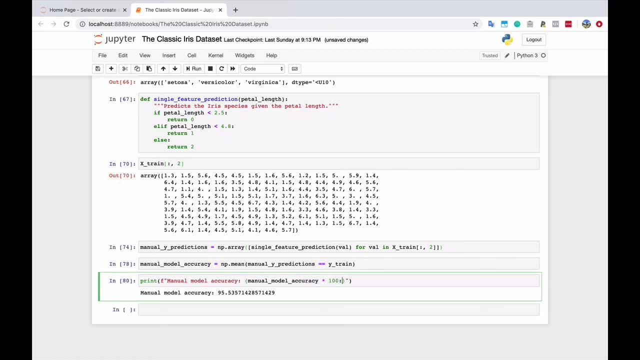 then we can format it by doing a colon and maybe I'll give it a, maybe I'll give it to, I'll give it two decimal places. so I'm saying, you know, give me a decimal place, give me two, two digits after the decimal place, and we're we're formatting. 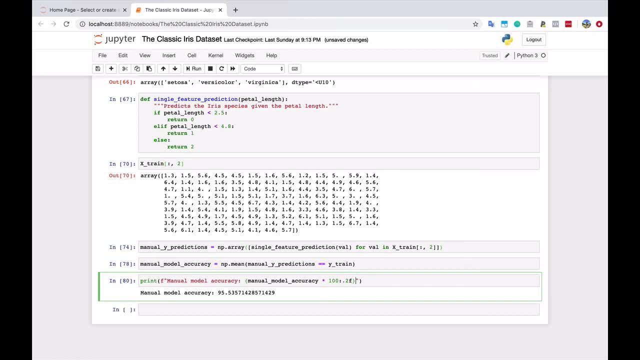 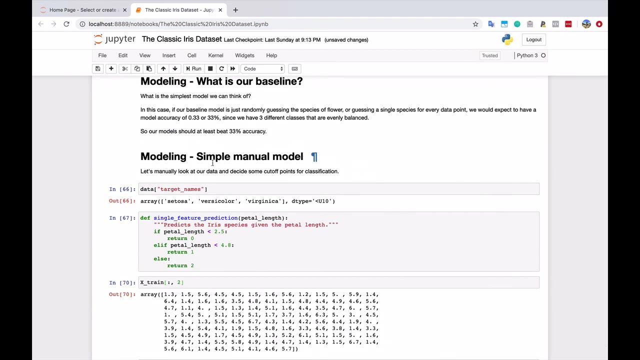 this is a float, which is what that F stands for, I believe, and then I'll add a percent sign kind of at the very end, just to format this as a percent, and so there's some nice formatting there for our model accuracy all right, and so that was pretty cool, this simple manual modeling, and I think 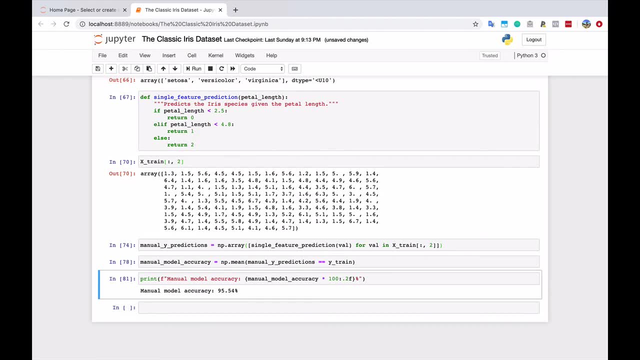 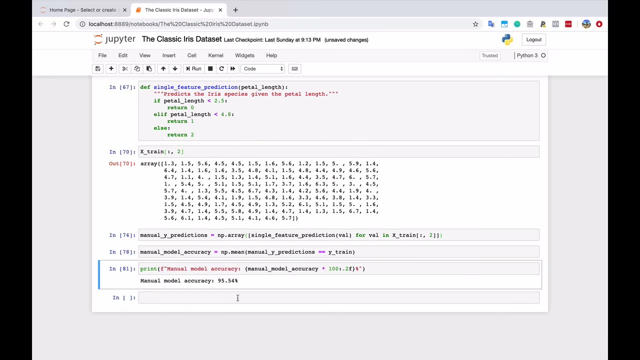 we're ready to move on to our logistic regression now and and so, even though we are able to get really good results kind of manually, we're gonna keep going and we're gonna show that we can get even better results using a logistic regression model. 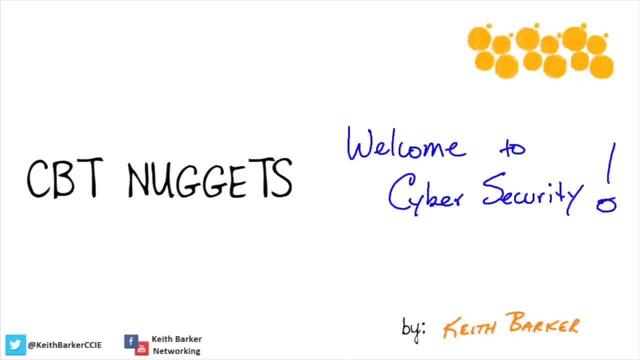 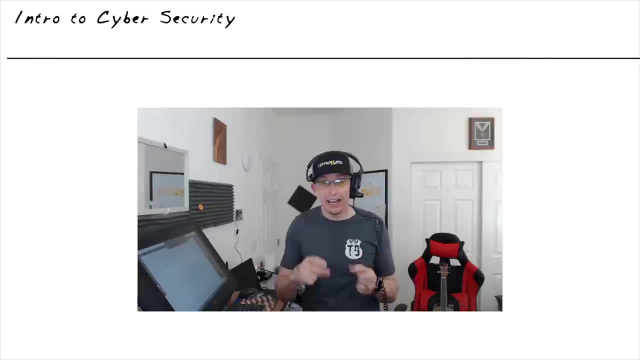 It was a Monday morning and I was digitally empty, meaning I had to leave my smartphone and laptop. anything digital I had to leave behind as they checked my clearance level and let me in. And it turns out that's the process that has to be followed when you're entering a secure area. And I thought to myself as I was working on those systems- whoa, back in the 80s I was a cashier and now I'm in this secured area working on some really amazing secure systems. How did this happen? And the answer is: it happens one step at a time.